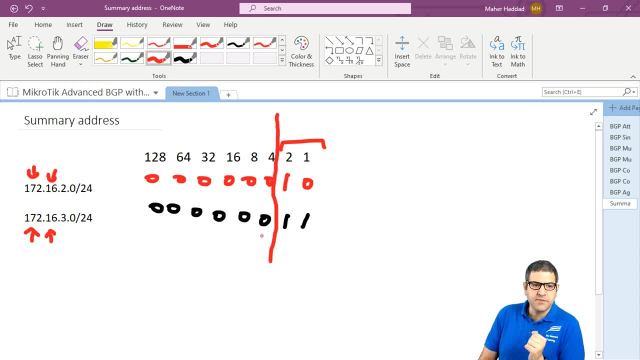 over here. So what does it mean here? This means that the summary address in this case is going to be 172 and 16 is the same. It's not going to change. So we put 172.16 is not changing. Now the third octet. you can see that we have here zero, So we have to put zero, dot zero, and the last octet is dot zero. So we see that all of those are zeros And the last one is also zero. You can see it over here. 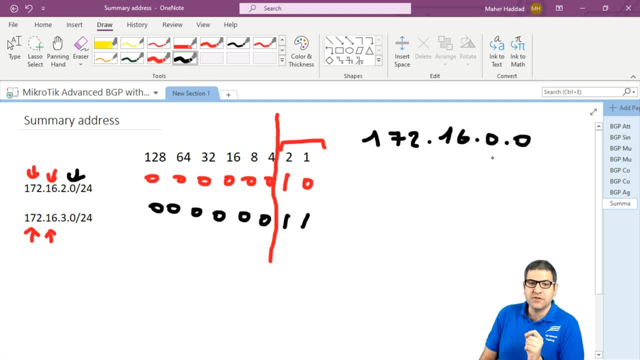 so we just put this one, 172.16.0.0. now what is the subnet mask? so you know that the subnet mask say for you if this octet is changing or not. so we see that 172 is not changing. so this is 8 bits, so 8. 16 is not changing on both addresses, so then also 8, so 8 plus 8, so we have 16. now those 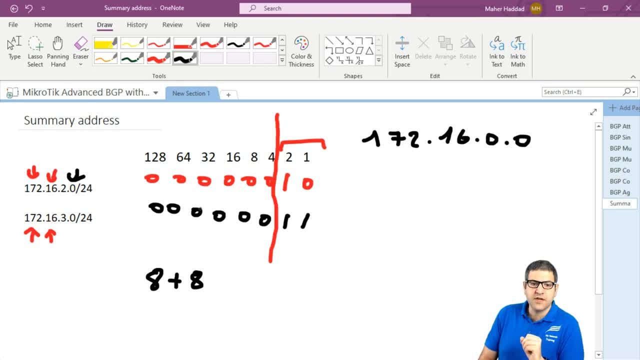 we are now on the third octet. you see that those zeros are not changing. they are the same. so we count them: 1, 2, 3, 4, 5, 6, so plus 6, and at the end the last one, because this is the. 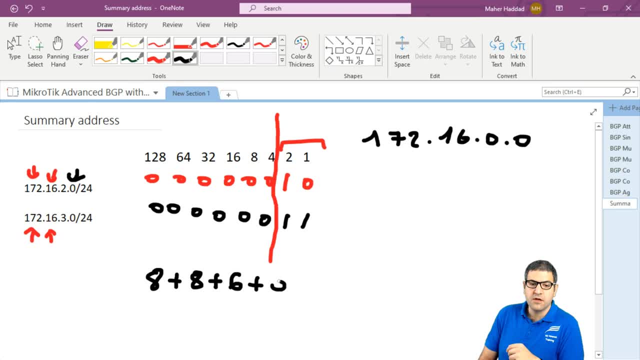 host. so it's gonna change. so then plus 0, then the subnet mask in this case is 8 plus 8, that's 16 plus 6, that's 22. so that means this. here is the summary address: 172.16.0.0.0. 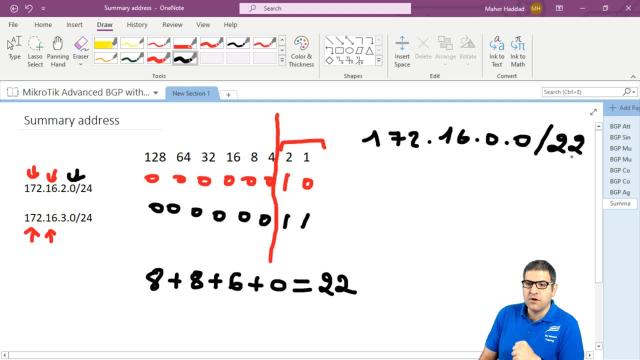 slash 22 and if you know or you want to know what is slash 22, so it is 255.255.25. in this case it should be 2.0. why 252? because we said that the first two octets are not changing, so this is 255. 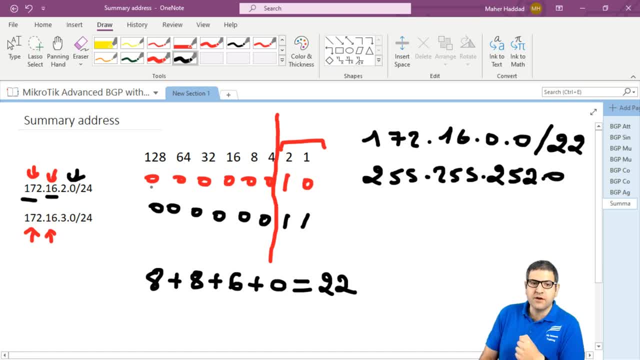 this is 255. now, what is not changing over here are those zeros. so we count them: 128 plus 64, that's 192 plus 32, that's 224 plus 16, that's 240 plus 8, 248 plus 4, that's 252, so this: 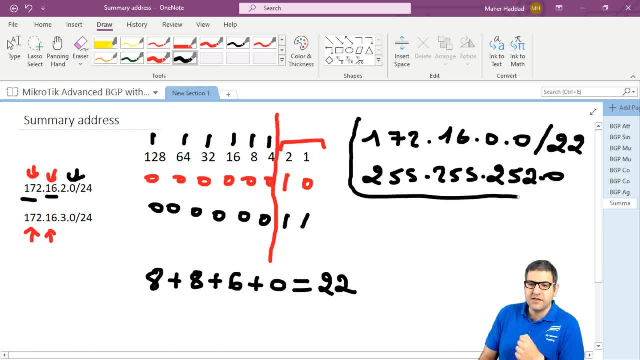 is really what is the result. so you can see that now this is the summary address. so in case you have, for example, two networks, that you want to do the summary for them. but also in case you have much more networks, that you want to do the summary for them. but also in case you have 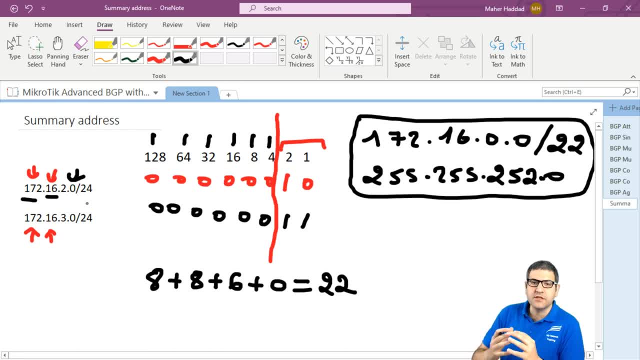 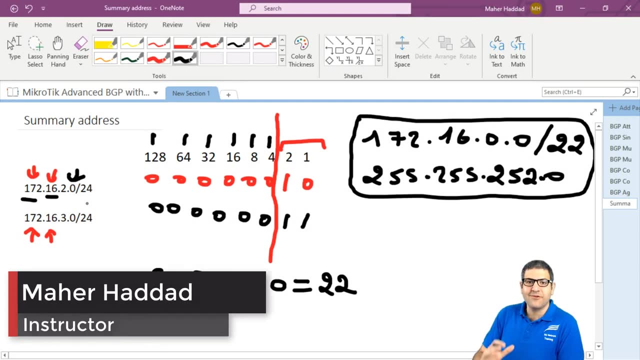 they have similarity somehow, then you can do the summary others for them and then at the end you will represent them with one prefix, and then this will take much less load on the cpu when you are advertising them to another router. so this is what i wanted to show you. now it's only about how to do. 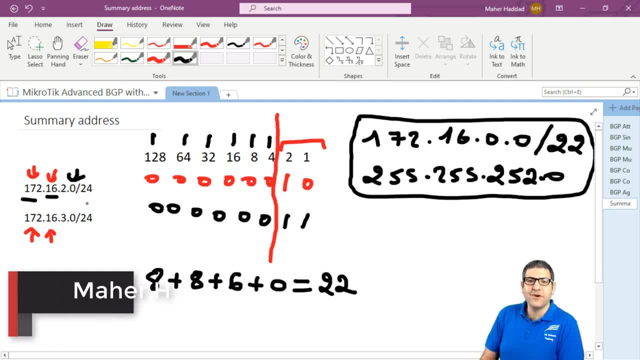 the summary, others. i hope that this video was informative for you and i will see you in other videos. 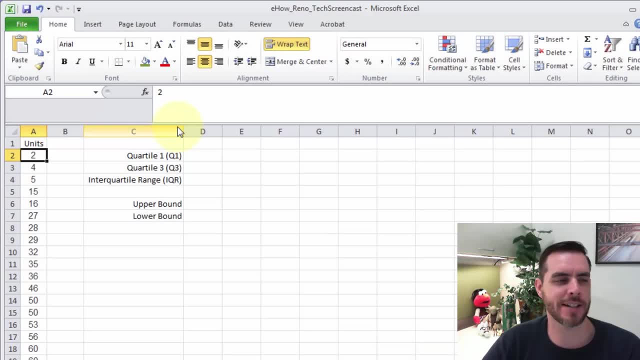 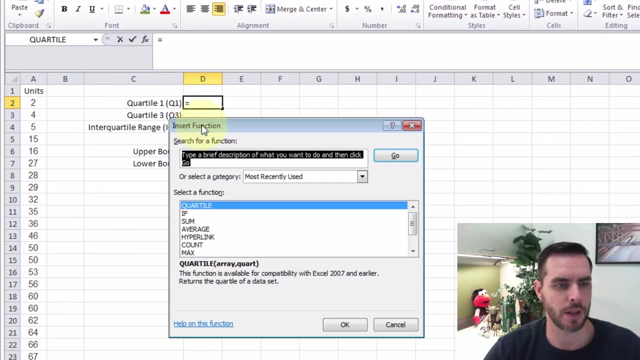 Let's figure out the outliers in your data set First. we can already take a look, and here's all the things we're going to be solving for. So first thing we want to do is get our first and third quartiles, and to do that let's click on the insert function button. Then we'll look up quartile and 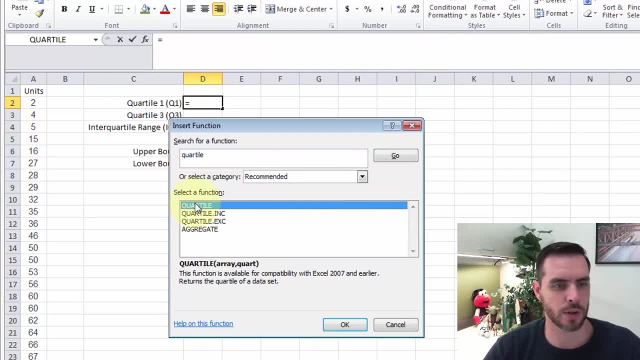 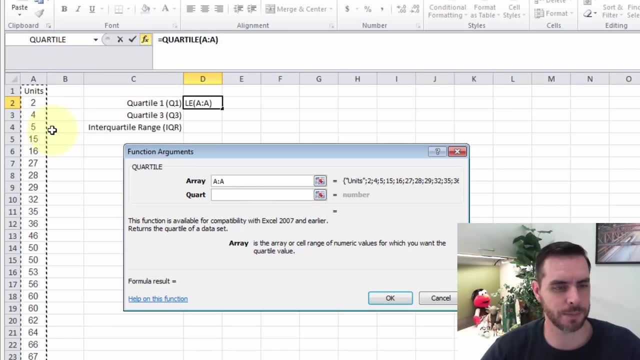 click go Here's quartile. we'll select it and click OK. Now we need to give it our array and we'll highlight this first column and we'll say we're looking for the first quartile and this will give you all the information here on what each number value means. So first we're looking.